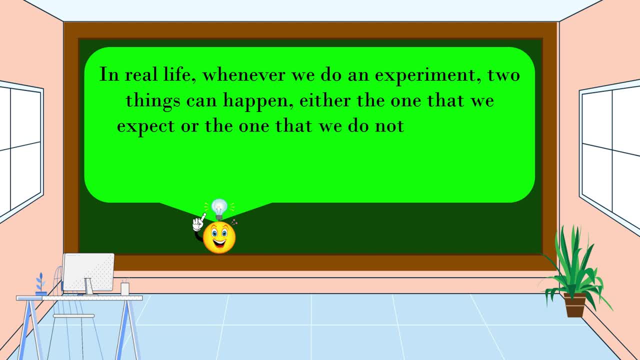 Is there the one that we expect or the one that we do not? When the result is what we expected, then it is the favorable outcome. Let's do an experimental probability using a spinner. Observe and watch the spin fortune and how it works. 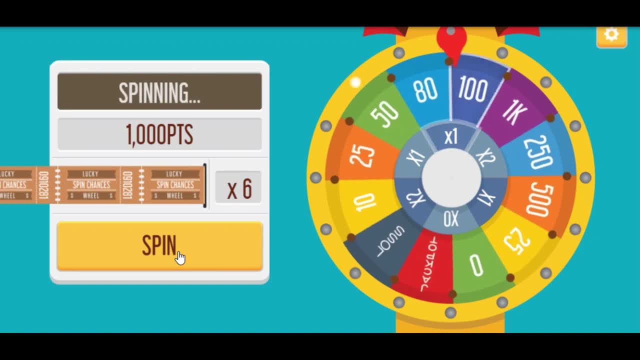 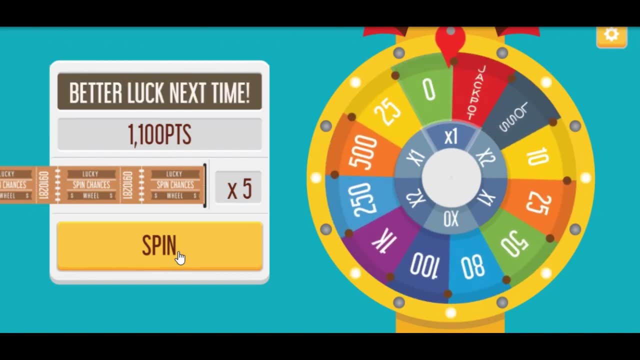 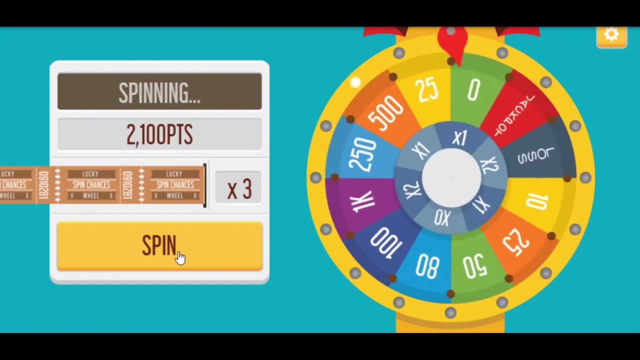 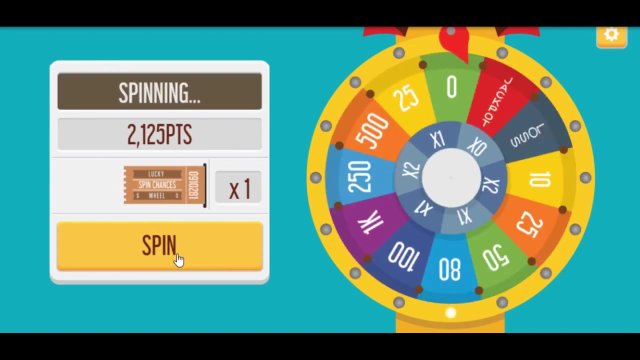 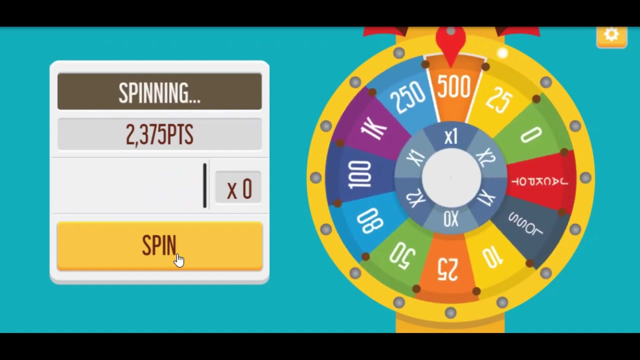 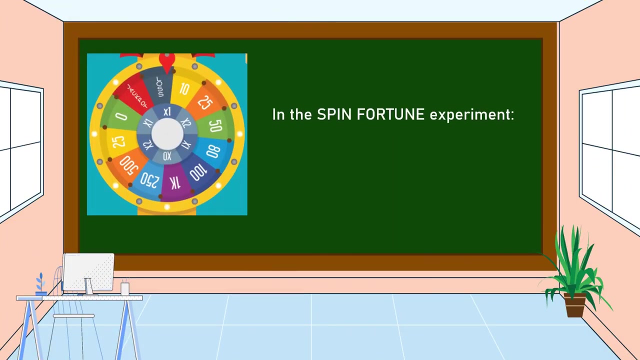 blowback Roll lead without a slide. 4 open 3 an. 3, 3, 3, 3, 2, 1, 0, 0, 0, 1, 0. deployment In the spin fortune experiment. what is the chance of picking up each element in the spin fortune wheel? 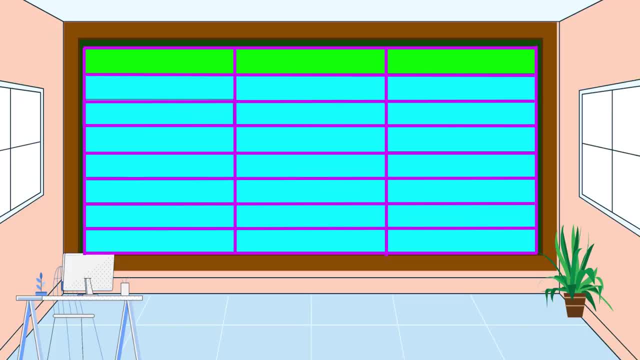 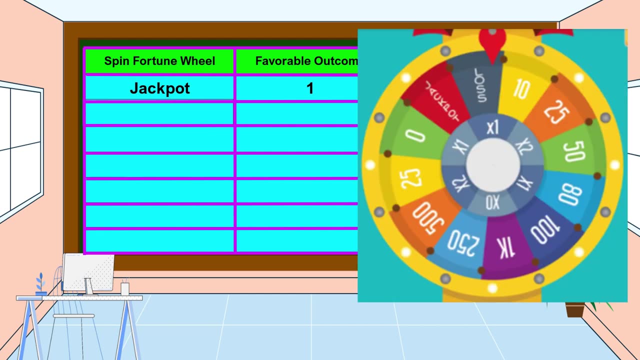 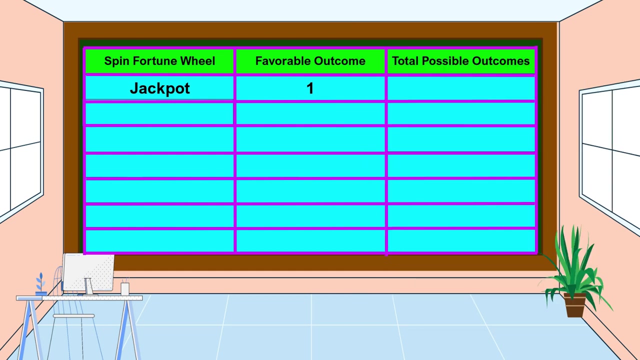 To know the answer, let's list down all the favorable outcome and the total possible outcomes For jackpot. the favorable outcome is 1.. As we can see in the spin fortune wheel, there is only one jackpot, so the favorable outcome is 1.. 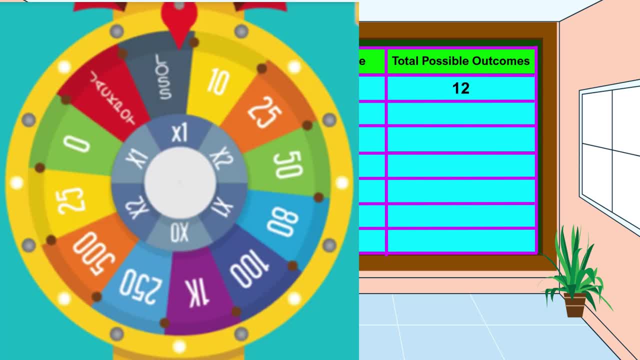 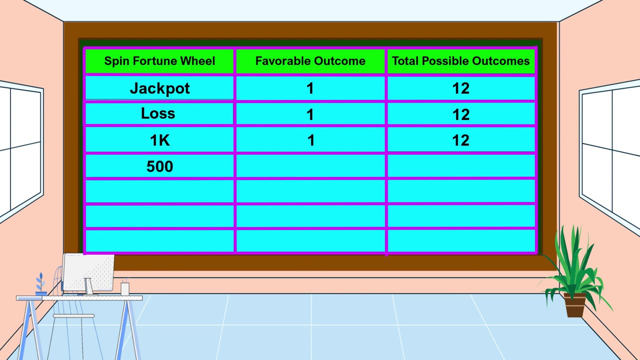 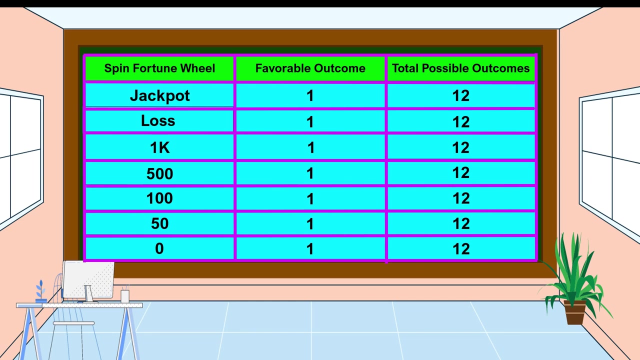 For the total possible outcomes? the answer is 12.. Why? It is because we will count all the elements in the spin fortune wheel, Same also with the other elements in the spin fortune wheel. These are all the favorable outcome and total possible outcomes in the spin fortune wheel. 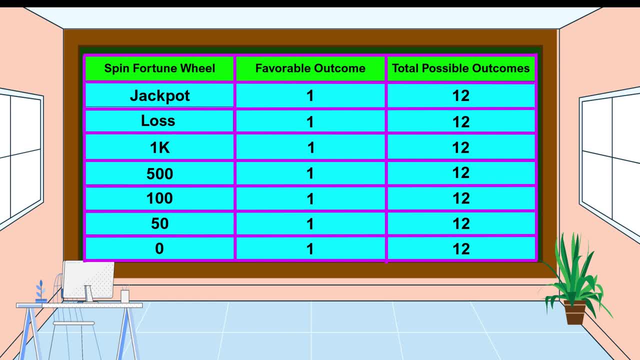 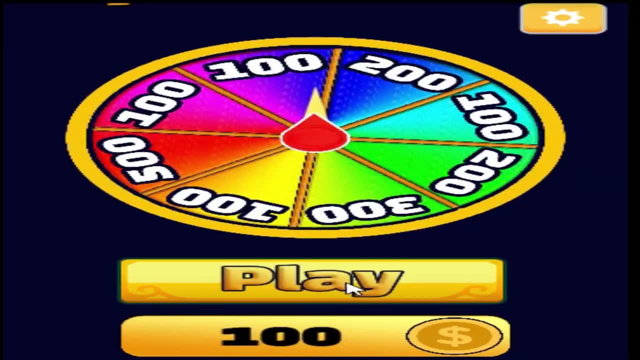 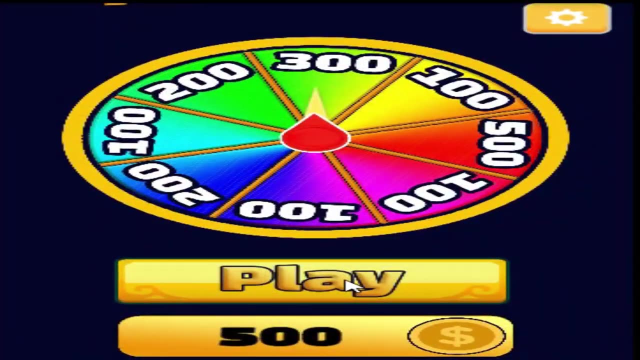 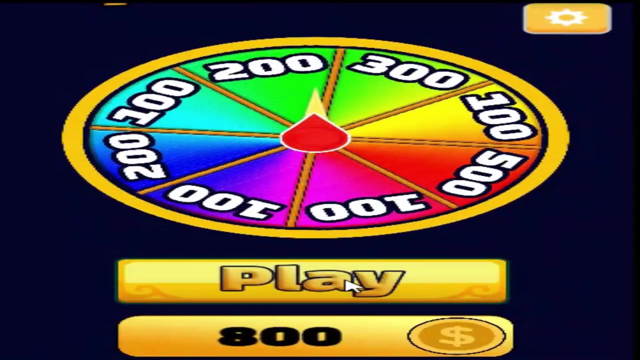 Let's observe and watch. another experimental probability. Let's have a look. The negative energy of the spin allowance is 1., The non-negative energy is 2. And the positive energy is 3. If we multiply the negative energy of the spin allowance with the positive energy of the sait. 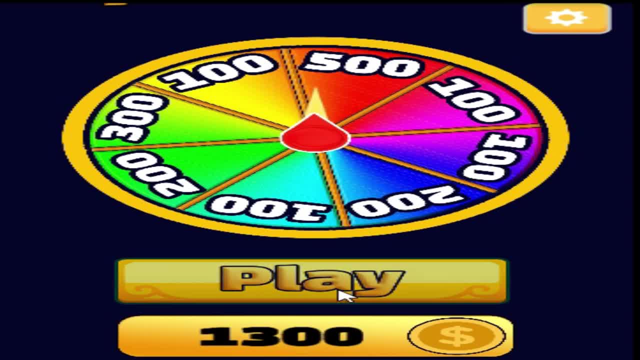 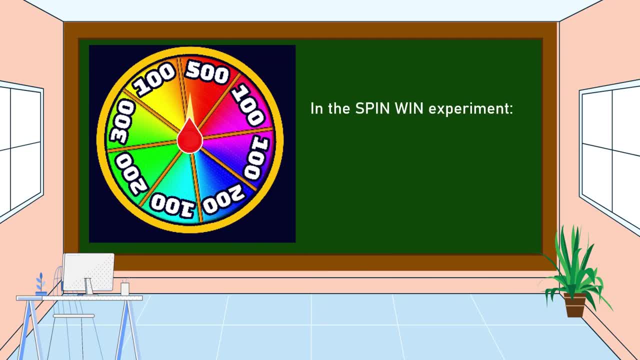 weattle and coirgelene will change its present and future form. Therefore, although these ambos are the non-negative and positive aspect in the spin fortune wheel, the Afterbirth expression of the spin is not in the spin fortune wheel. In the spin-win experiment what is the chance of picking each element in the spin-win wheel? 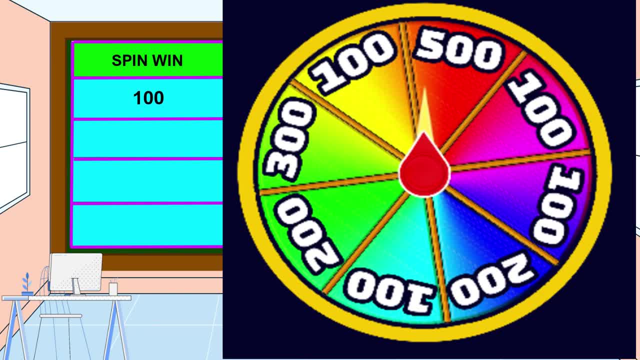 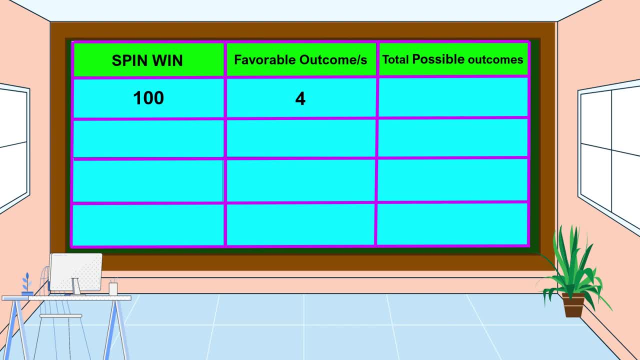 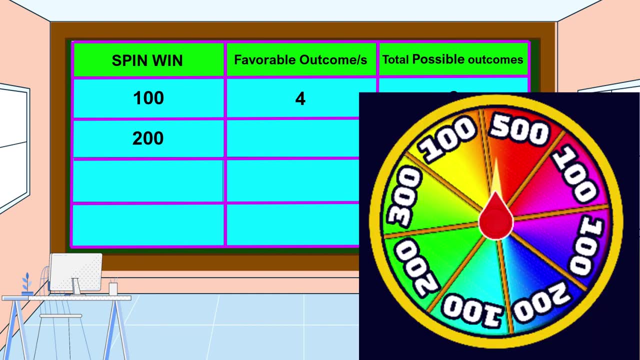 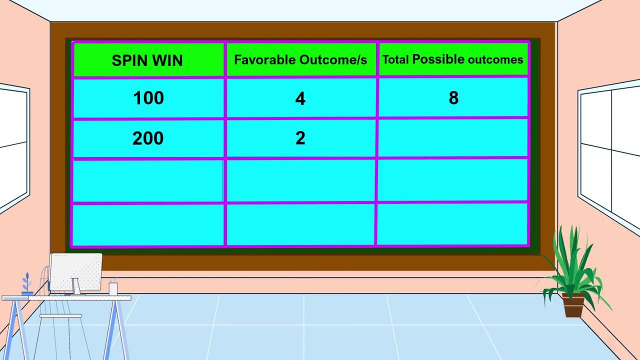 Since there are 4 100 in the spin-win wheel, then the answer for favorable outcomes is 4.. The answer for total possible outcomes is 8.. There are 2 200 in the spin-win. therefore, the answer for favorable outcomes is 2 and for the total possible outcomes, the answer is 8.. 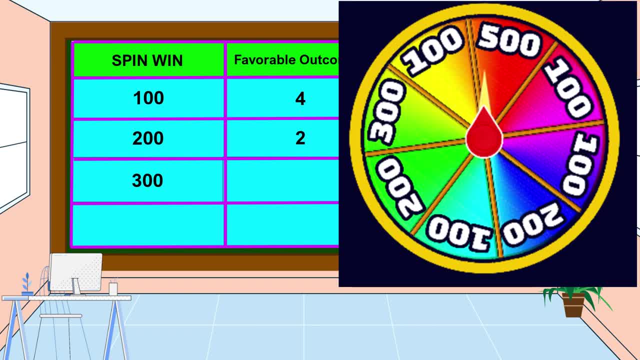 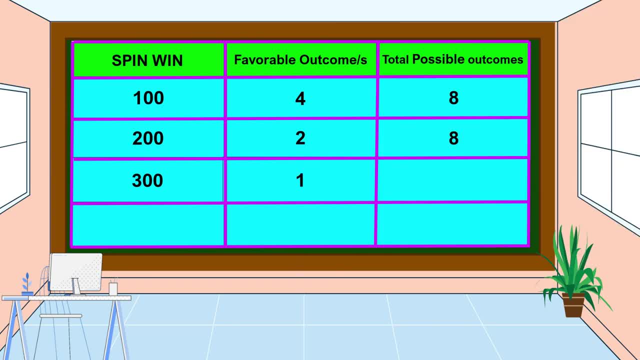 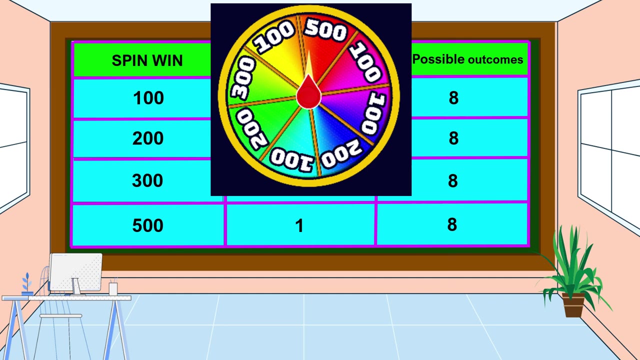 For 300, there is only 1 300 in the spin-win. so the answer for favorable outcome is 1. And for the total possible outcomes, the answer is 8.. Likewise with 500, there is 1 favorable outcome and 8 possible outcomes. 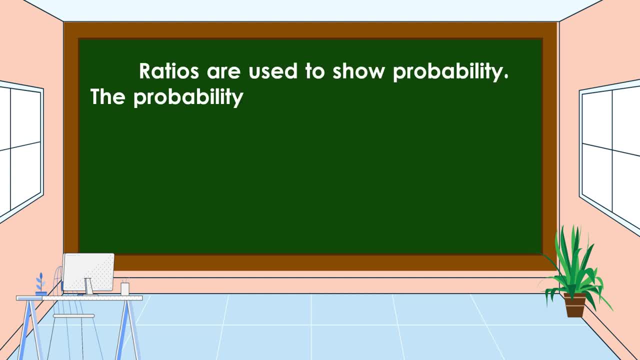 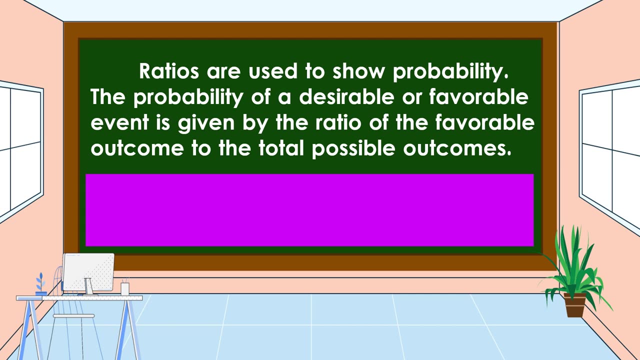 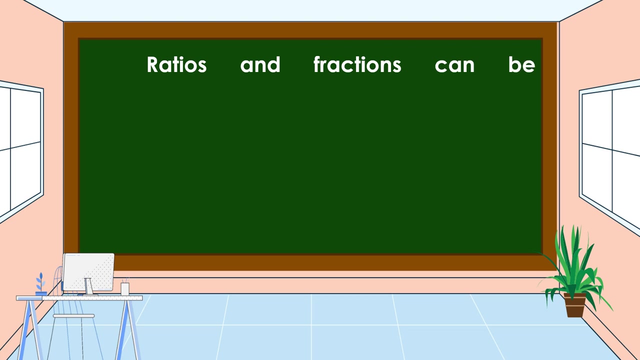 Ratios are used to show probability. The probability of a desirable or favorable event is given by the ratio of the favorable outcome to the total possible outcome. This is our formula: Probability of an event is equal to favorable outcome over total possible outcomes. Ratios and fractions can be expressed in simplest form. 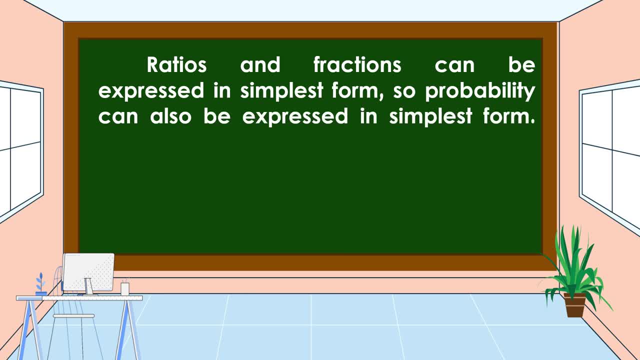 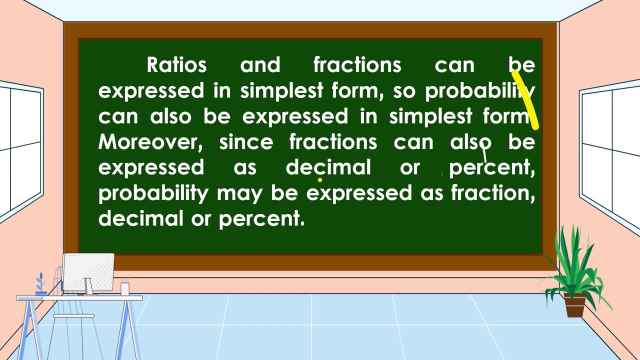 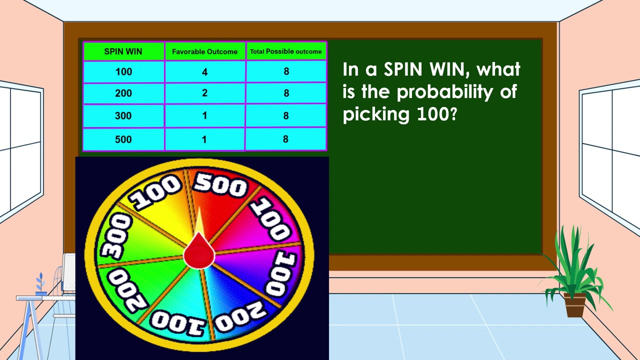 So probability can also be expressed in simplest form. Moreover, since fractions can also be expressed as data- decimal or percent- probability may be expressed as fraction, decimal or percent. In a spin-win. what is the probability of picking 100?? What is the formula? how to find the probability? 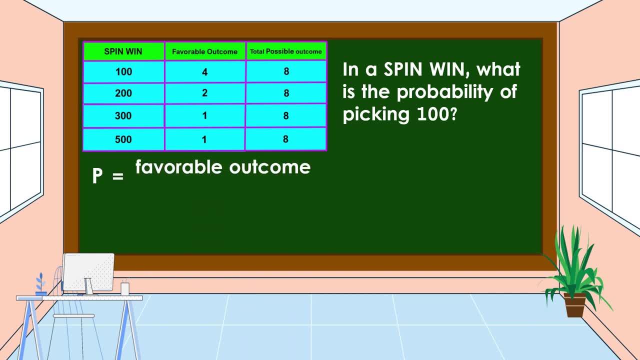 Yes, you are right. P is equal to favorable outcome over total possible outcomes. So in our chart, favorable outcome for 100 is 4 and the total possible outcomes is 8.. So let's reduce 4x8 to its lowest term. 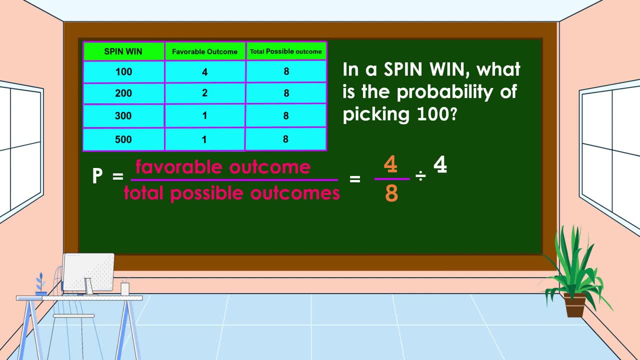 4 and 8 are both divisible by 4.. 4 divided by 4 is equal to 1.. 8 divided by 4 is equal to 1.. 8 divided by 4 is equal to 1.. 8 divided by 4 is equal to 2.. 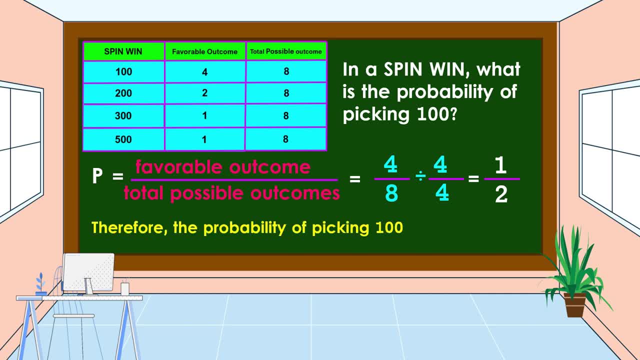 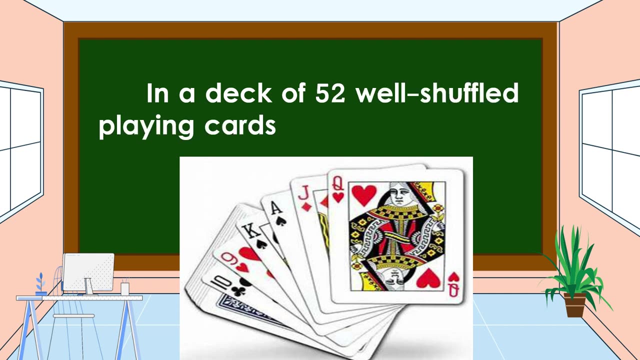 8 divided by 4 is equal to 1.. Therefore, the probability of picking 100 is one half or 50 percent. Another example: In a deck of 52 well shuffled playing cards, what is the probability of getting a queen? 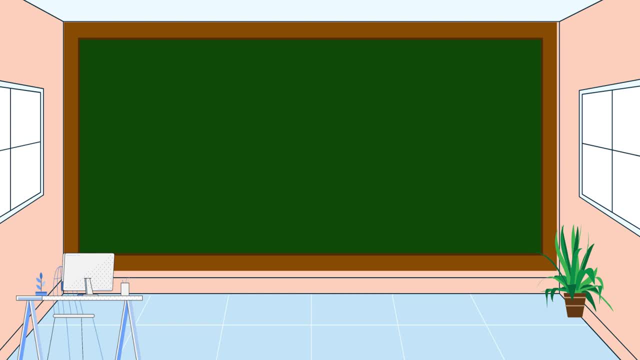 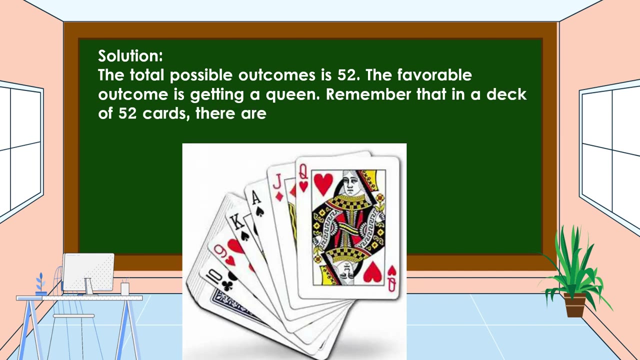 What is the probability of getting a queen? This is our solution. This is our solution. The total possible outcomes is 52.. The favorable outcome is getting a queen. Remember that in a deck of 52 cards there are 4 suits and each suit has a queen. 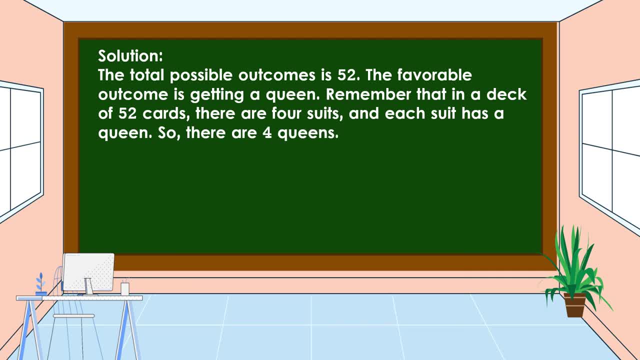 So there are 4 queens. What is the formula? how to find the probability? Alright, the formula is: Probability, or P is equal to favorable outcome over total possible outcomes. So the favorable outcome is 4 and the total possible outcomes is 52.. 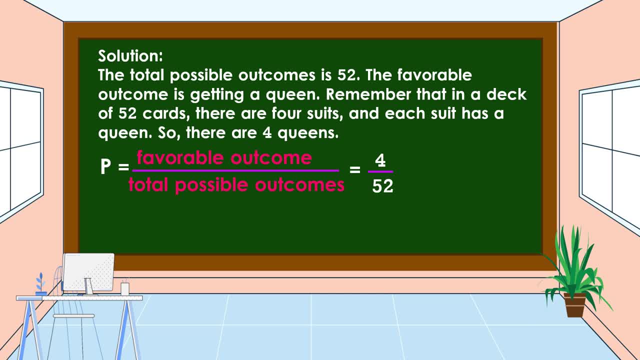 Then let's reduce to its lowest term 4 and 52.. 4 and 52 are both divisible by 4.. So let's divide: 4 divided by 4 is equal to 1.. 52 divided by 4 is equal to 13.. 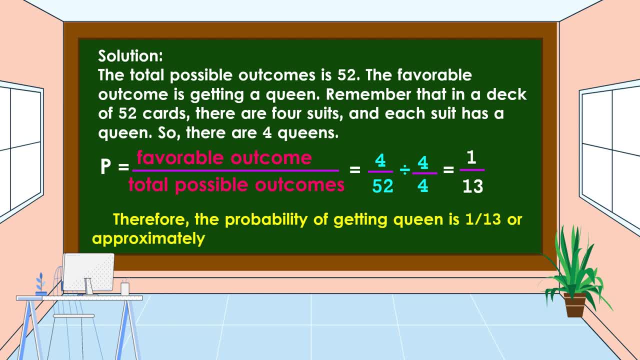 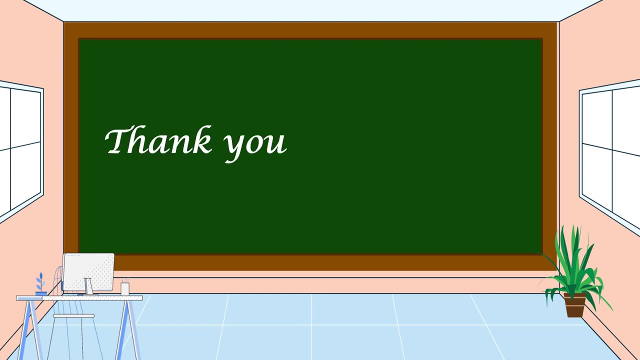 Therefore, the probability of getting queen is 1 over 13 or approximately it is 77,000 or 0.077.. I hope that you understand our lesson for today and thank you for watching Subtitles by the Amaraorg community.